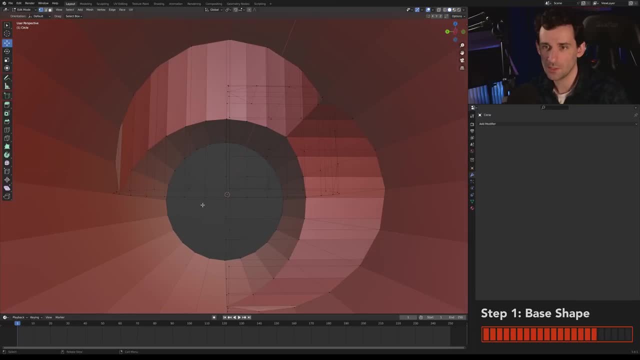 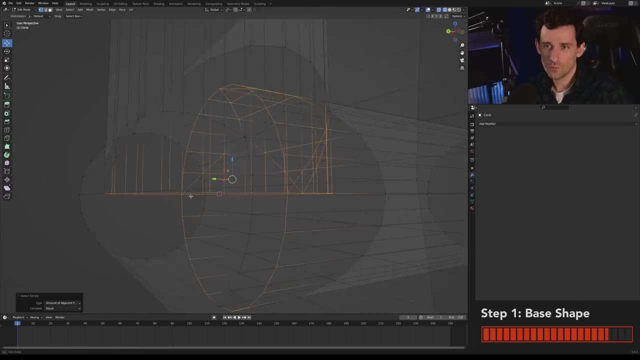 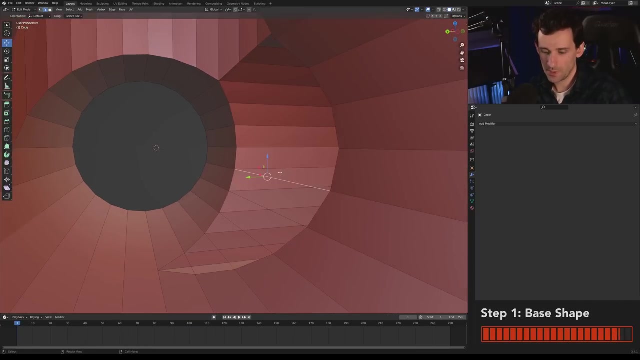 Alt H to unhide the rest of the geometry. And to clean this up, let's select one of the vertices. Shift G: amount of adjacent faces. Now we have all those loose vertices selected. Let's delete them, And we need to repeat the same steps for those loose edges here. So I'm going to select one. 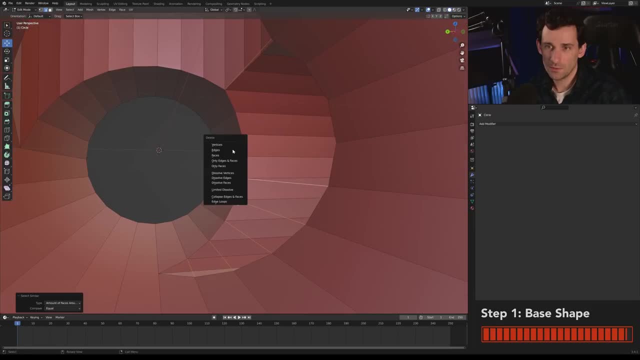 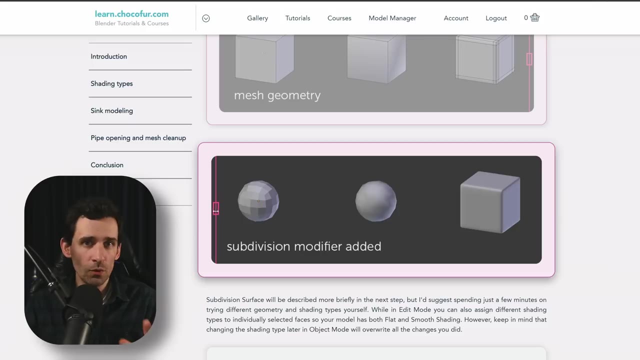 Shift G: amount of faces around an edge. Let's delete those, And now we have a perfect base shape to start working with. Throughout this video, I'll be using the good old, quite often forgotten subdivision modeling technique, which basically means: 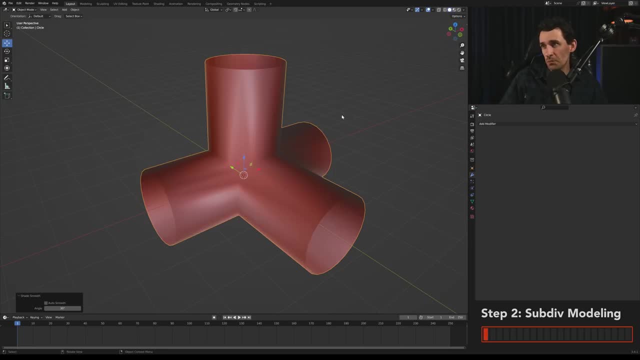 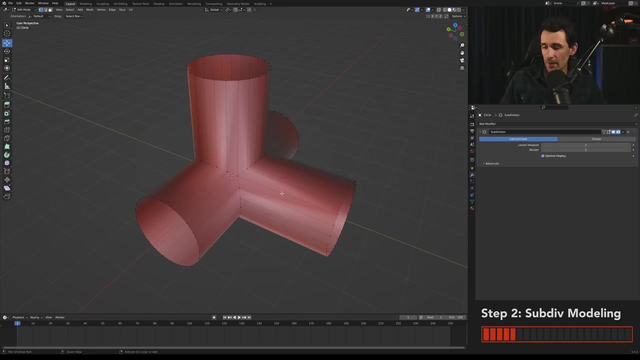 two things. First, when I change the shading of my geometry to smooth, this doesn't happen. And when I apply a subdivision surface modifier, this doesn't happen. So with this object the solution is quite simple. We enter the edit mode, disable the subdivision surface modifier. and now I just press Ctrl on it And now we have a perfect base shape to start working with. Throughout this video, I'll be using the good old, quite often forgotten subdivision modeling technique, which basically means two things: First, when I change the shading of my geometry to smooth, this doesn't happen. And when 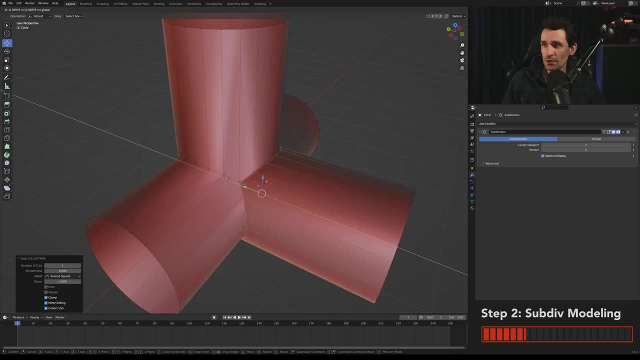 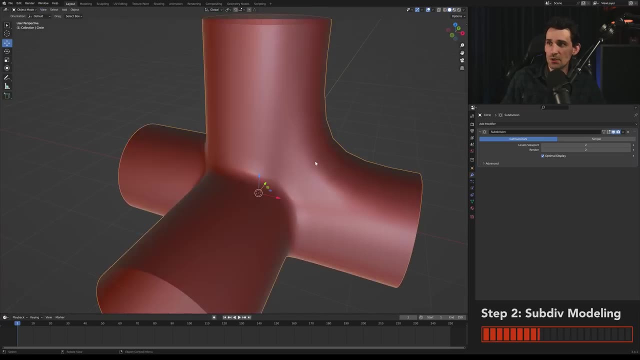 I apply a subdivision surface modifier, this doesn't happen. And now I just press Ctrl on it And now I just push it back a little bit. Now let's do the same here And I'm just gonna keep this side untouched. So now, when I exit the edit mode, you can see the difference. So this extra edge loop. 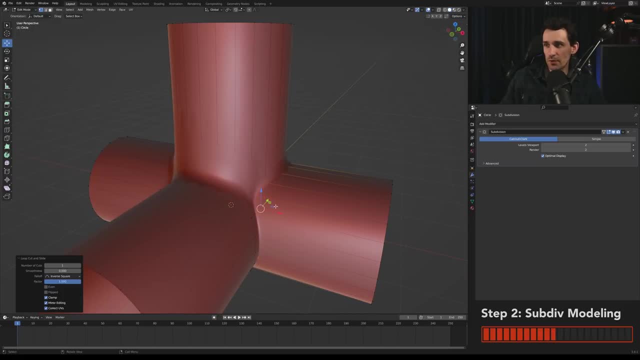 when I press Ctrl R, you can see how it affects the geometry. I always need to move it back. don't do stuff like this, because you're gonna get killed by somebody- in the professional environment, of course, And now, or in Minecraft. 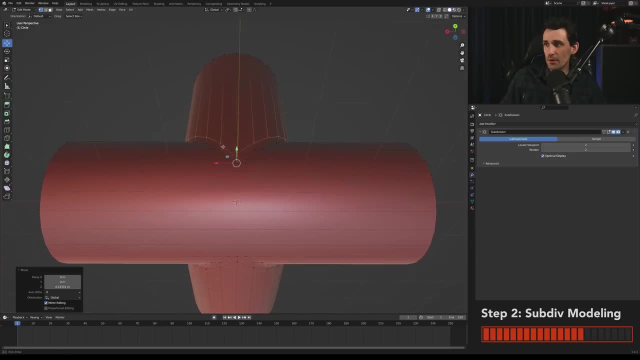 and now I'm going to move this extra edge here And here in the back. the problem: we didn't add the extra edge loop. that would prevent us from having those shading issues. So the way to fix it is simply adding an extra edge loop here by using the knife tool. 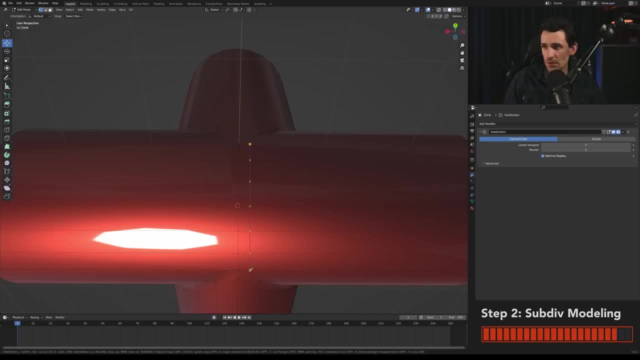 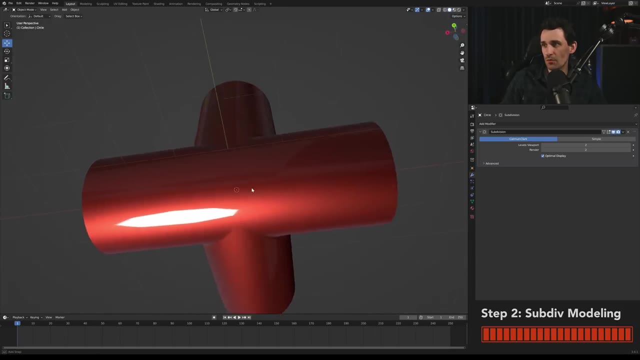 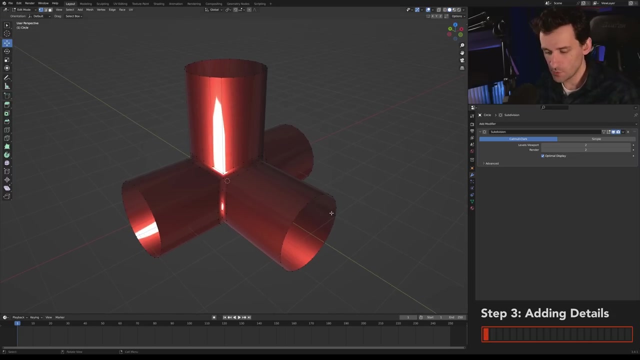 I should have actually done that before. I've added those edge loops. If you make the same mistake, fear not. just add three extra edge loops here And this already fixes the entire geometry. So to have an actual pipe, we still need to add some thickness to it. The easiest way is selecting. 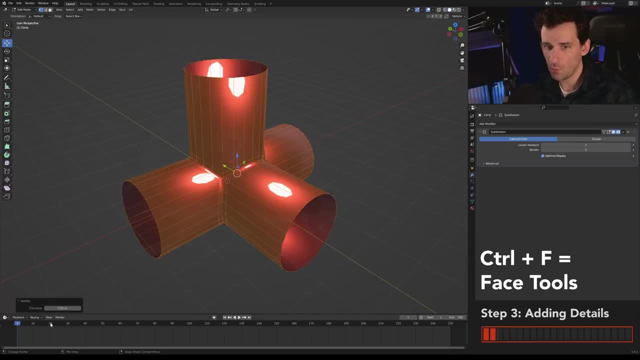 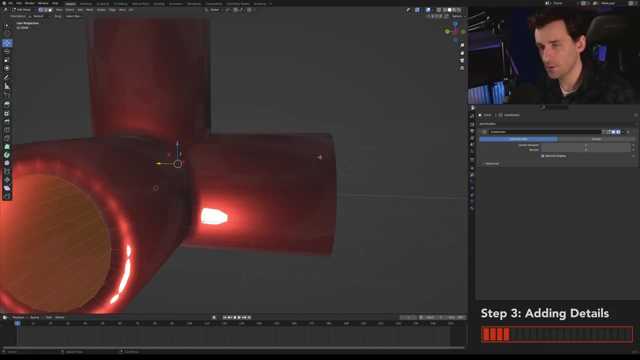 everything, pressing Ctrl F and choosing the solidify faces tool. However, I'm going to show you a little trick. As soon as you add it, you can see the subdivision surface modifier is rounding the endings of our pipe, which can be fixed, of course, by adding the edge loops like this. But now, 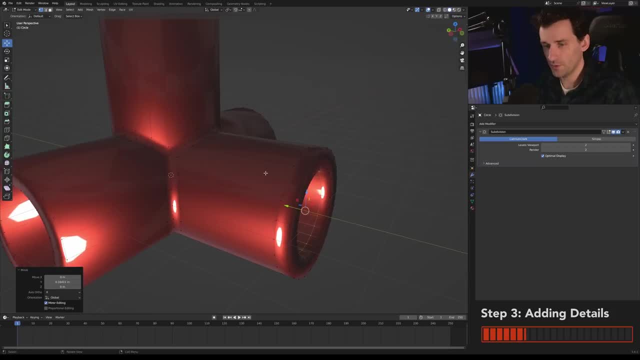 you also have to do it on the inside. So let's avoid the unnecessary work And before you apply the solidify faces, we're going to do the same thing on the inside. So let's avoid the unnecessary work And before you apply the solidify faces, 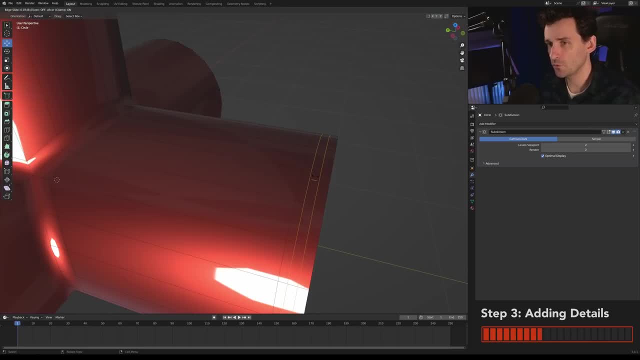 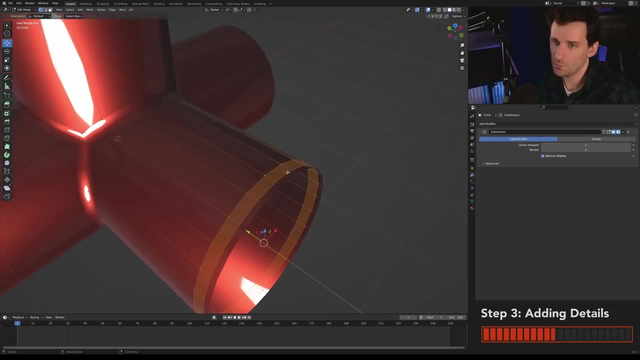 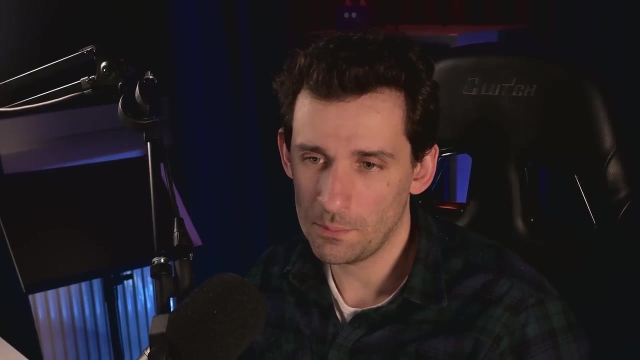 just add the edge loops before that. The way I like to do this on the edges of the model is adding this extra support loop here. So this way I'm sure both the geometry and shading of my model will stay perfect every single time. All I have to do is applying the solidify faces again. but to make 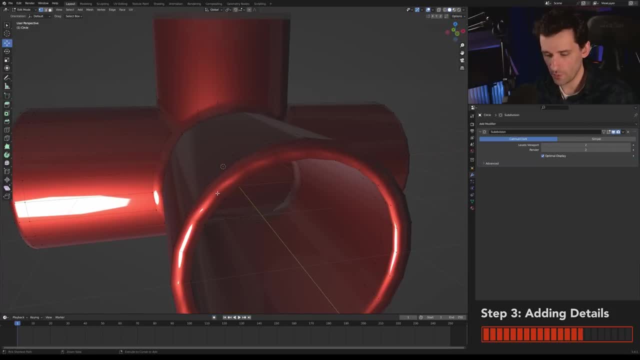 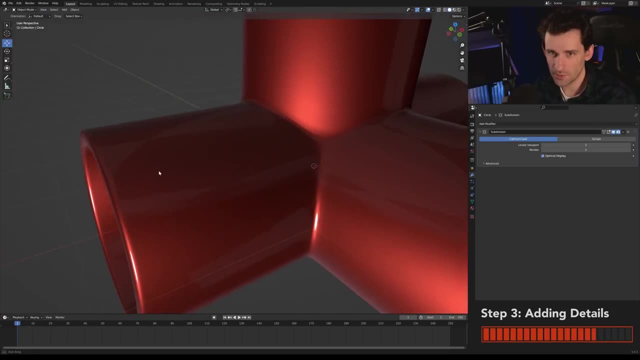 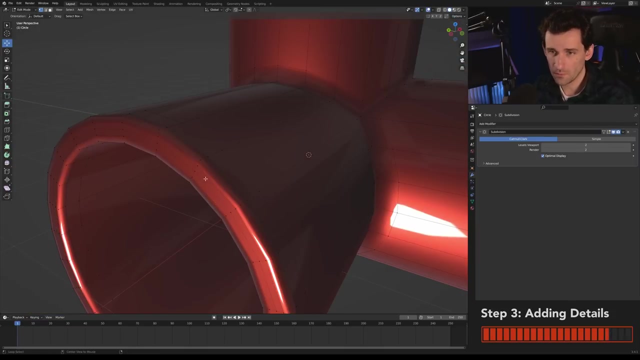 the model absolutely perfect so we can show it to anyone. You need to add three edge loops here, And if you look at the model you can see that the edges of the model are a little bit rounded. So unless this is the effect you want to achieve, you can keep it, But I always add those extra edge. 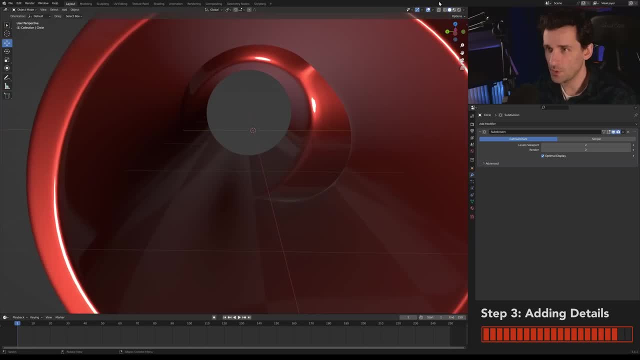 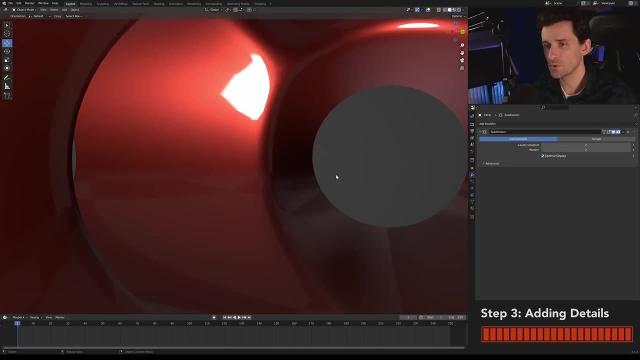 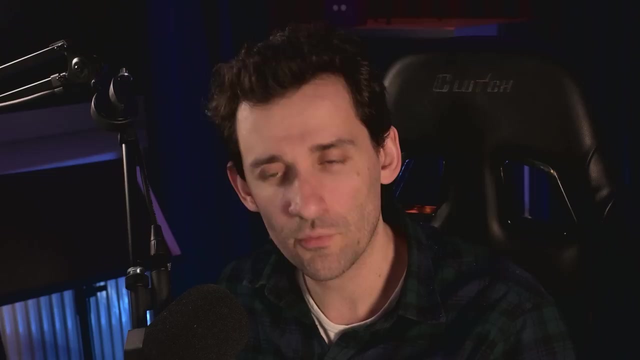 loops so it looks pristine. What's also amazing, when you look inside the model, we have all those pretty shapes preserved. So if you show it to someone you know, 3D mesh tells a lot about a human being. If it's done right on the inside as well, everyone will respect it. 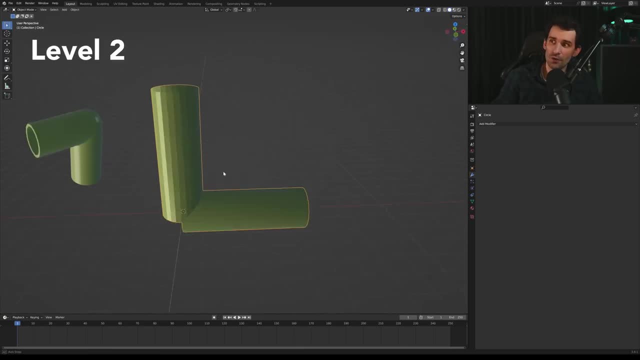 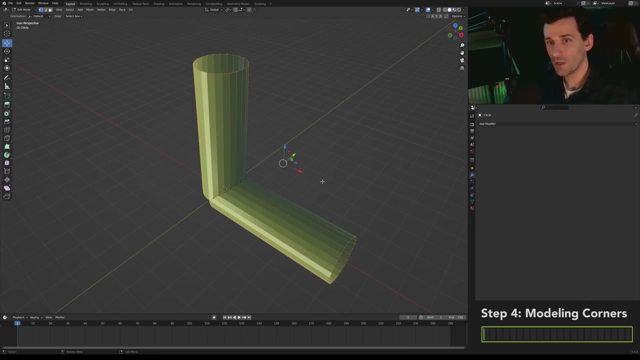 Now this second example is actually way harder than you think, And before you go into comments and write how stupid my method is, go ahead and try it, because what we are doing here is will be actually. Before we begin. I have a little confession to make. Turns out with those. 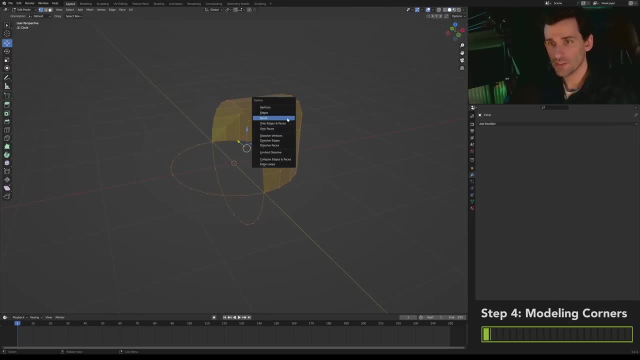 booleaned objects, you can actually go ahead and delete the faces. This is my 3D artist excuse, but I really didn't know that. However, to my defense, if you do it this way, you can't add edge here, And that's because you need to remove the doubled vertices. Select everything with A key. 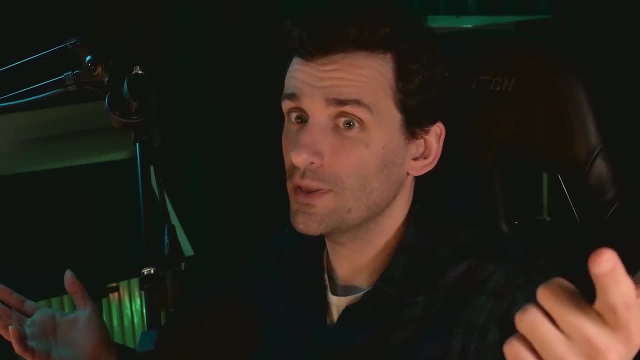 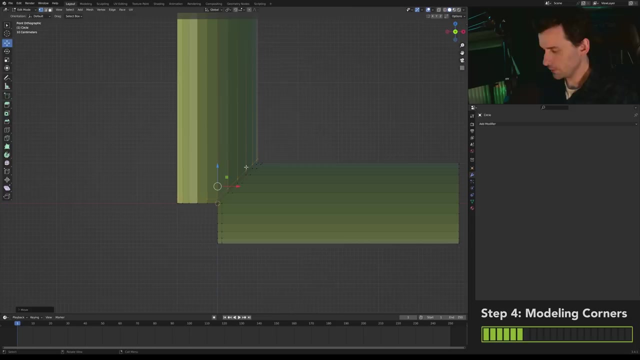 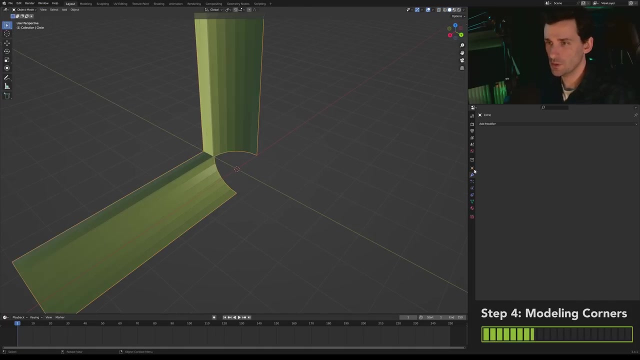 press M and choose by distance. Hey, you know two methods now. I will now add two edge loops next to each other and close to the main edge here, And I'm going to delete actually half of this model and use the mirror modifier because we will have to do certain adjustments on both sides. 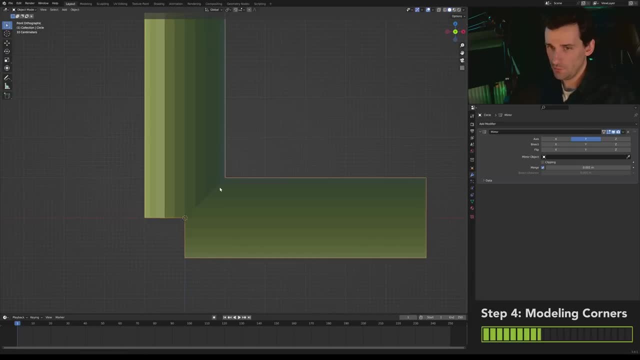 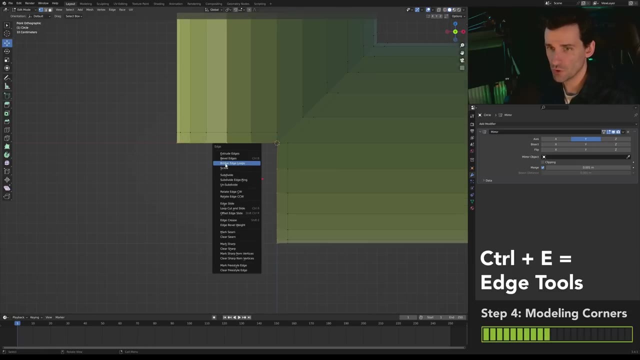 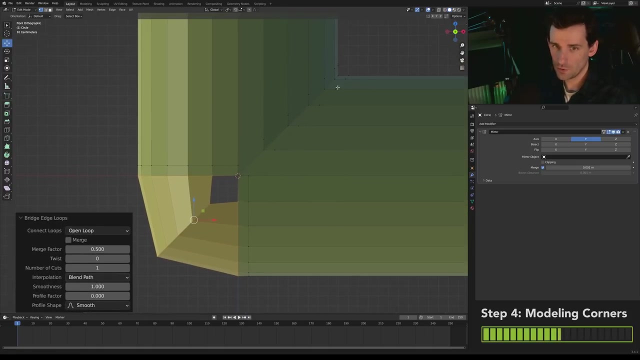 So let's just save ourselves some work. And now in the side view, I will select this edge loop. deselect the corner vertex. press control E and choose the bridge edge loops option here. Open up this window here. Add one more segment. This new segment corresponds to the main edge here. 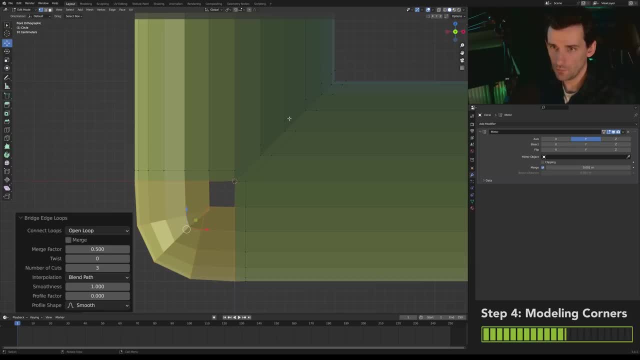 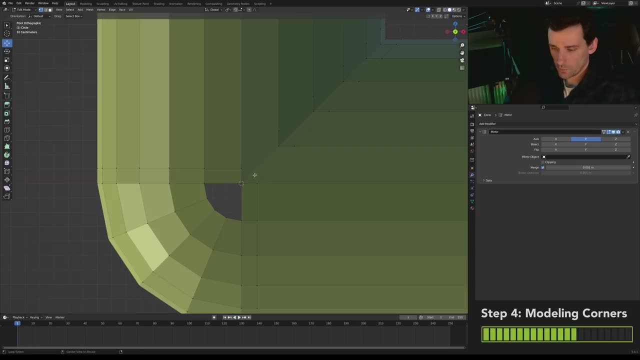 If we add two more segments, they will be corresponding to those edge loops. You can use this smoothness slider to fix the model, And what we want to do now is pressing the K using the knife tool and extending those edge loops. What we have to do now is filling those. 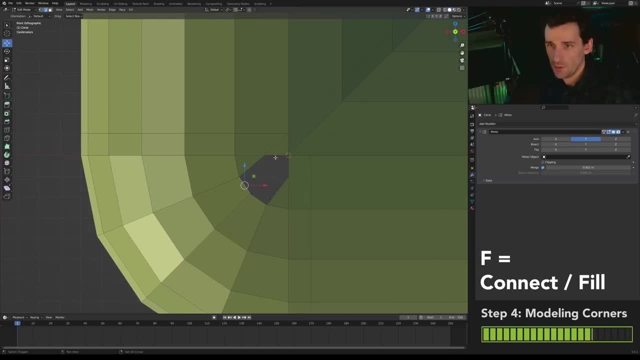 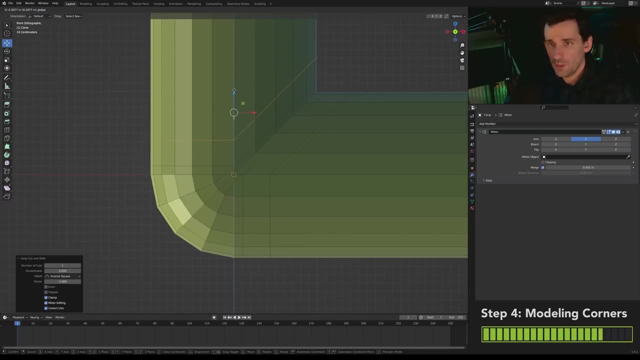 vertices. So I'm selecting the pairs of edges and pressing the F key to do it very quickly. Now we add two more edge loops, offset them a little bit further from the center And we also need to delete these edge loops. You can see we now have pairs of triangles here, So I'm just selecting. 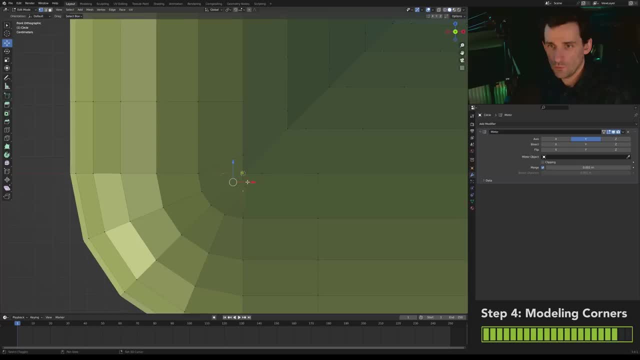 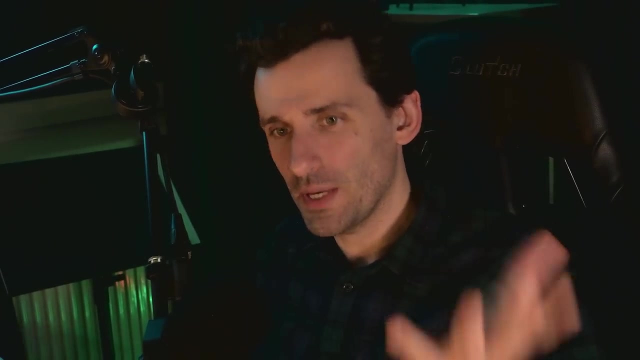 them and pressing F to convert them to quads, And I have to remove those two vertices by merging them into the last one. So I'm pressing M and merge at last. Now you can see. we have two more triangles here and here And a quad that we can create here. Now this model is basically done. However, I need to add: 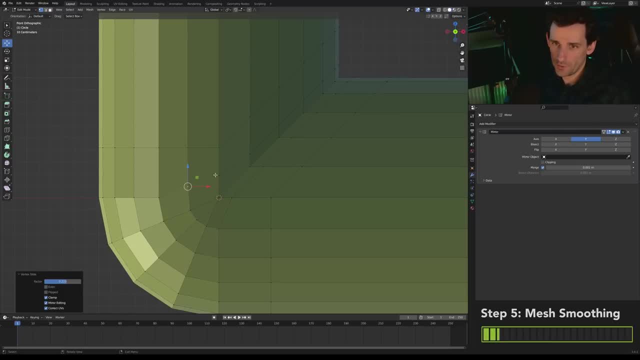 a little bit more curvature to this edge loop we have in here. So I'm just selecting the individual vertices, pressing G twice and aligning them along those main edges. Be sure to move those vertices along those edges, not like that. However, the most important vertex is this: 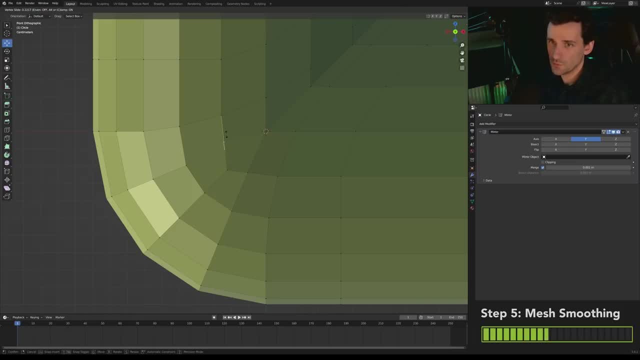 one in the end. I'm just going to pull it further from the center And those two vertices. these are the only ones you can actually move like that, but only slightly. You just want to make it smoother And this usually fixes absolutely all the shading issues. So, press. 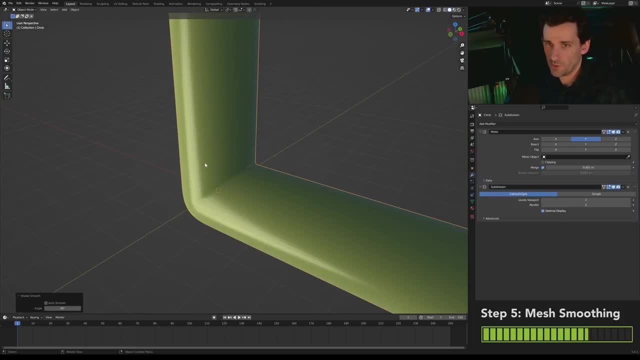 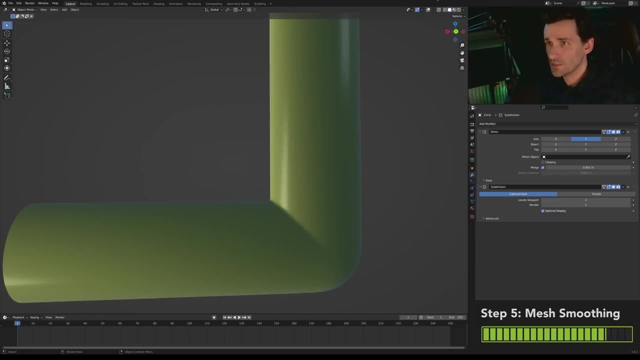 control two in the object mode to apply subdivision surface modifier, change shading to smooth. And come on man, tell me if you ever got a better and cleaner result than that, especially when you consider we have the 90 degree angle in here. I really tried many ways and wasn't able to come up. 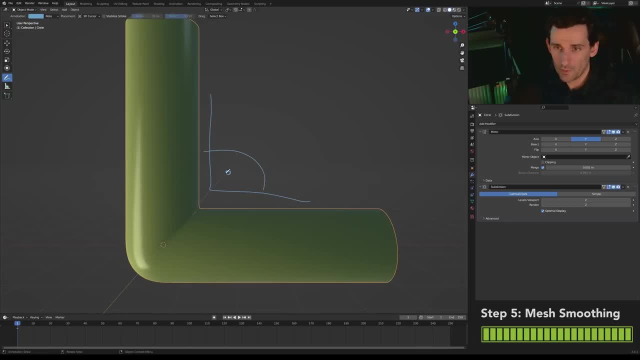 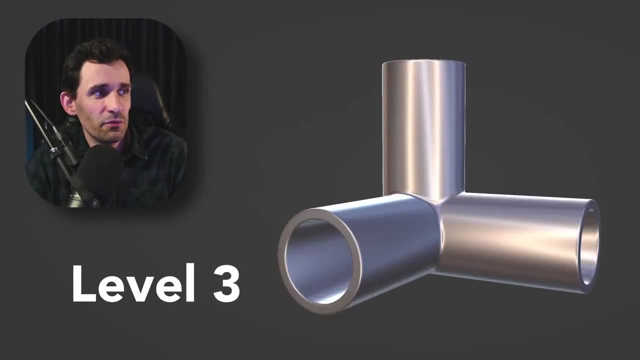 with one. So if you know the way, leave it in the comments. I would really like to try it out Now. the last object are three pipes joined under the 90 degree angle, And it's something I'm a little bit afraid of posting. the way I solve this It's quite primitive, quite unintuitive. So if you 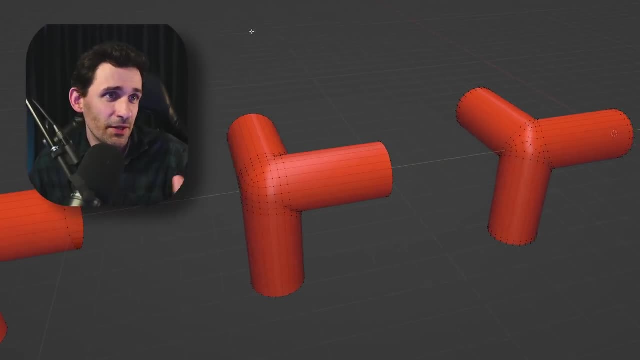 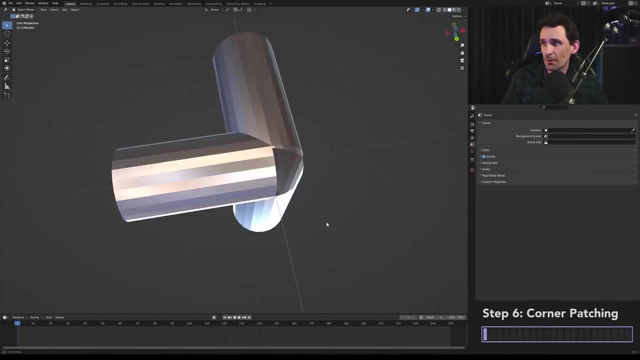 know a better way. feel totally free to roast me in the comments, because I've tested a few methods and I'm really curious: how would you guys do it? So we already have the base geometry in place and I'm going to add a UV sphere, So now I need to. 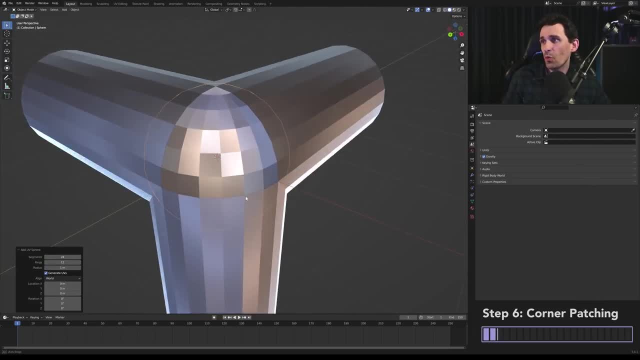 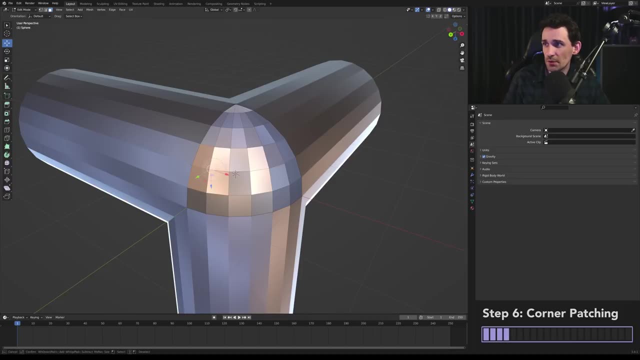 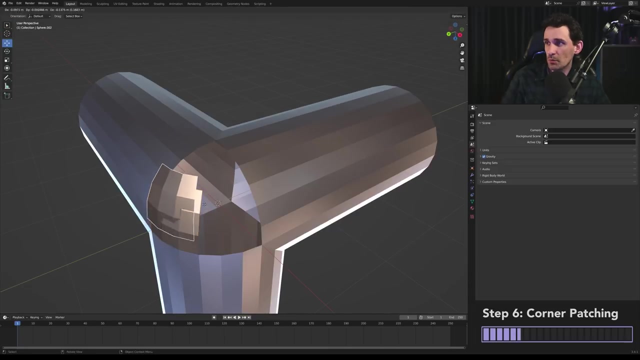 adjust it to our cylinders, our pipes, And what we want to do is using this corner for every single corner of our geometry. So I'm just going to enter the edit mode, press C and select those faces P to separate them And I'm going to delete the rest. duplicate and rotate within the X axis by 90. 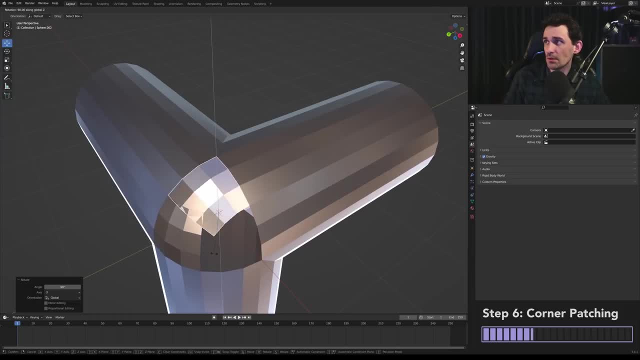 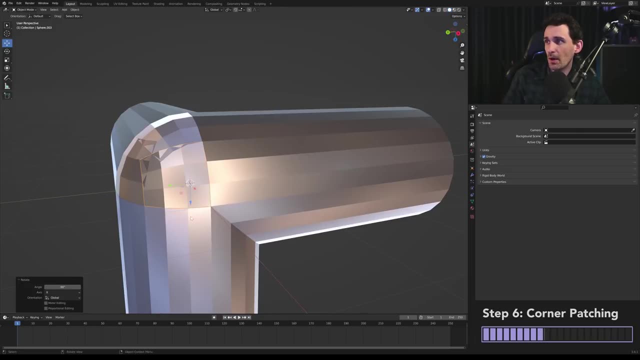 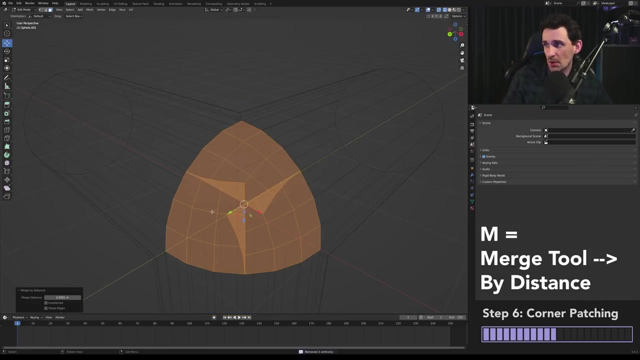 degrees, and now by Z axis by 90 degrees. Now I'm going to copy it again: rotate in Y axis and in the X axis by 90 degrees. And now we have to join those three parts together, Enter the edit mode, select everything and remove doubles. What we have to do right now is merging these. 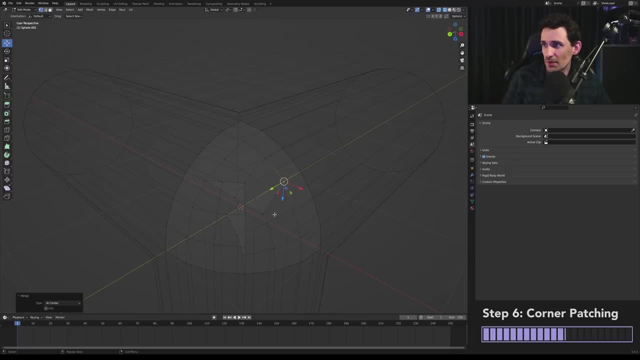 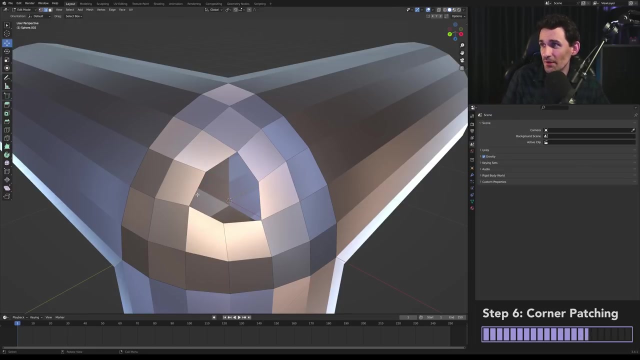 vertices at center. And what's primitive about this method? I guess you can already see. but what's unintuitive? First we have to delete these vertices. What's unintuitive is that the shape is completely without symmetry, but it works. I don't know what to tell you. It gives me the 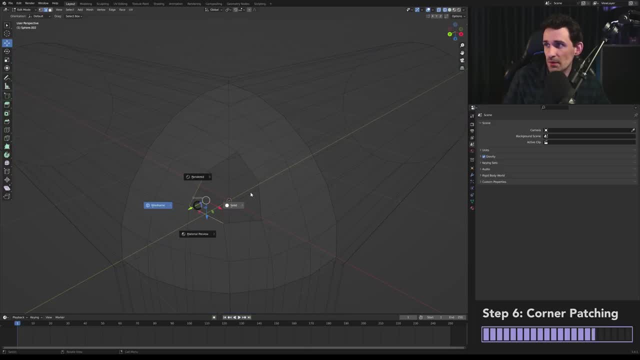 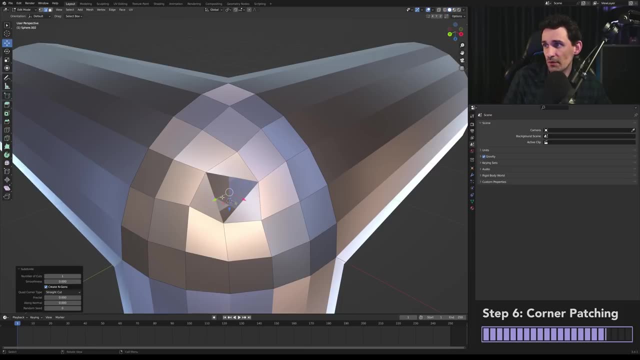 best result every single time. So now you can see I've reduced all of the vertices And now I'm going to create triangles here. I'm going to select these edges, right click and subdivide them. I'm going to now select all those vertices in the middle and join them at center. Now I have. 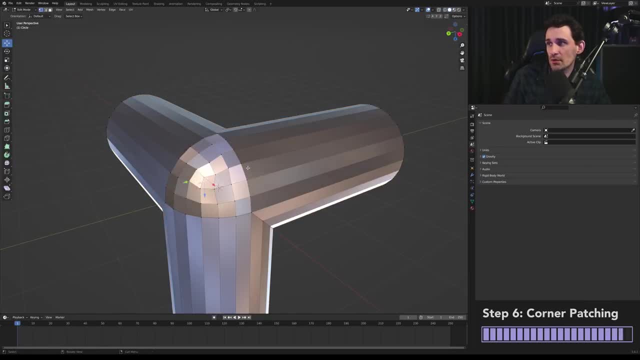 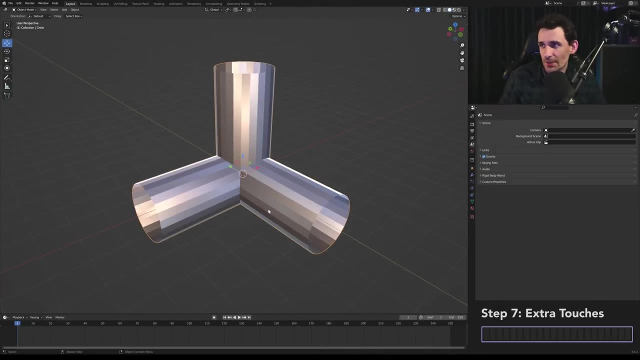 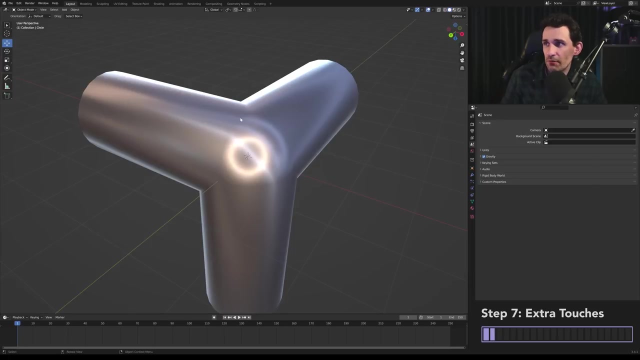 to select this mesh. join them by pressing control J, enter the edit mode, select everything, remove doubles and shift N to flip the normals. So let's preview the model. I'm going to apply the model to the model, add the edges, and then I'm going to add the edges. So the edges are. 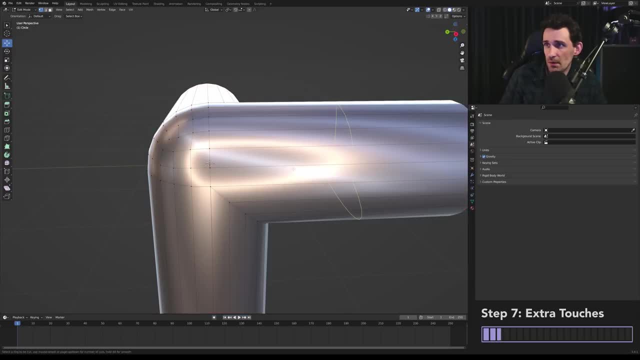 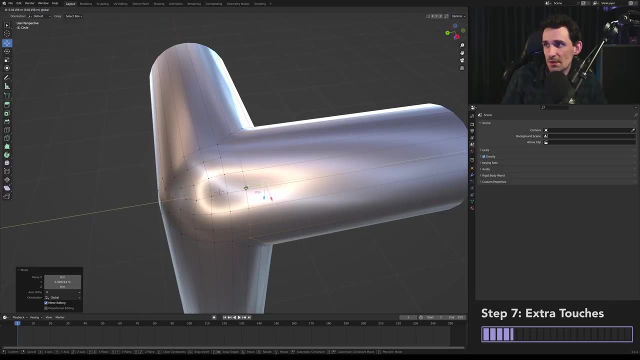 already smooth And you can already see it looks, in my opinion, perfect. right, We have those edges here, but we will remove them by adding the edge loops, sliding them to the limit and offsetting, So those squares are more or less the same size as those here in the corner. I'm going to repeat.